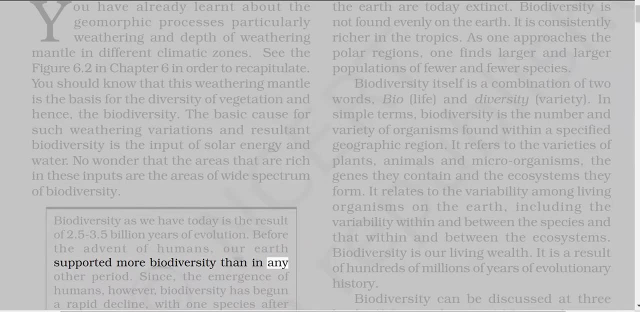 the advent of human birth, theunter created Об眾i, the coronavarii, 83 of them had created humans. our earth supported more biodiversity than in any other period Since the emergence of humans. however, biodiversity has begun a rapid decline with one species. 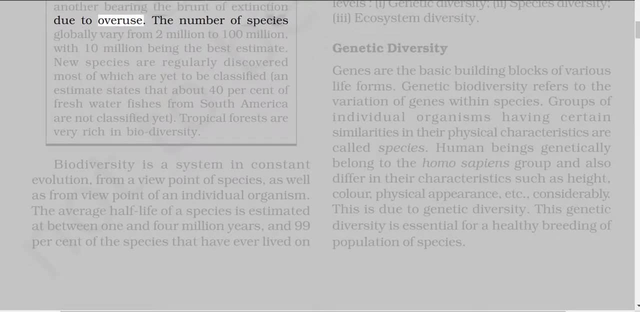 after another, bearing the brunt of extinction due to overuse. The number of species globally vary from 2 million to 100 million, with 10 million being the best estimate. New species are regularly discovered, most of which are yet to be classified. an estimate: 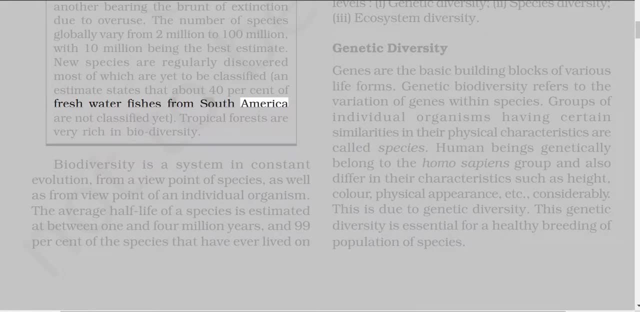 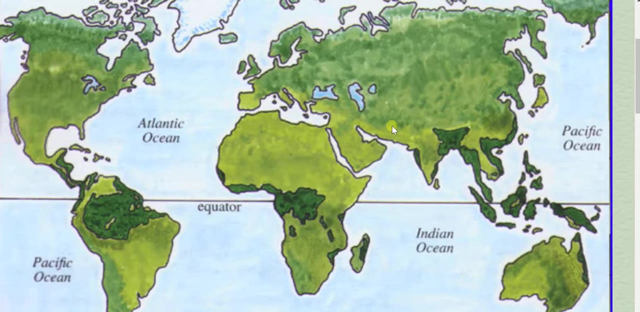 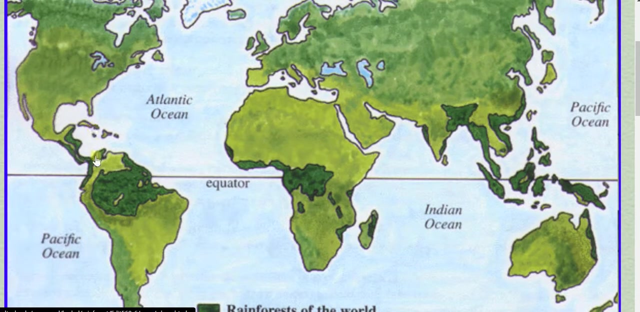 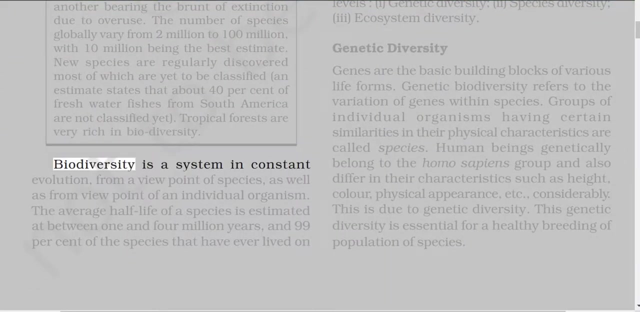 states that about 40% of freshwater fishes from South America are not classified, yet Tropical forests are very rich in biodiversity. Biodiversity is a system in constant evolution, from a viewpoint of species as well as from viewpoint of an individual organism. 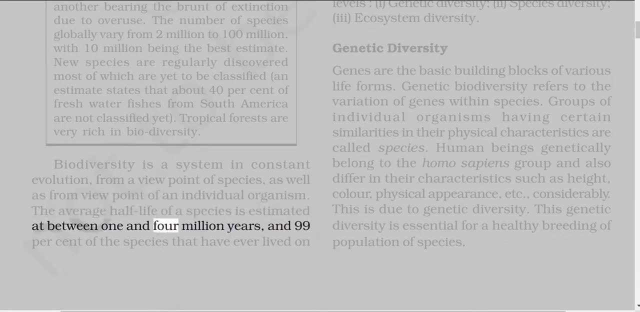 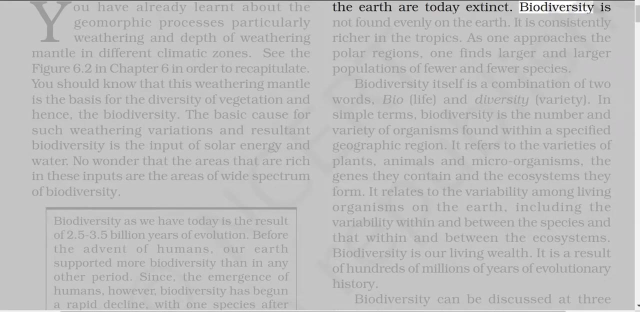 The average half-life of a species is estimated at between 1 and 4 million years, and 99% are of the species that have ever lived on the earth or today extinct. Biodiversity is not found evenly on the earth. It is consistently richer in the tropics. 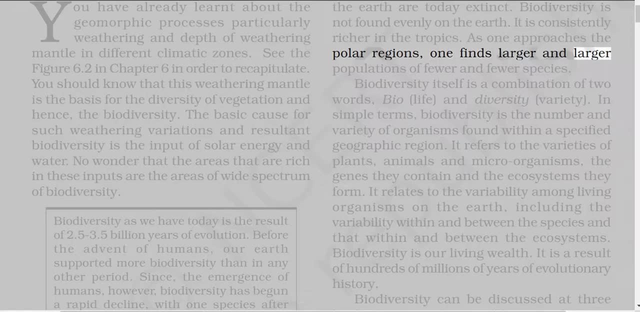 As one approaches the polar regions, one finds larger and larger species. There are larger and larger populations of fewer and fewer species. Biodiversity itself is a combination of two words: bio life and diversity- variety. In simple terms, biodiversity is the number and variety of organisms found within a specified 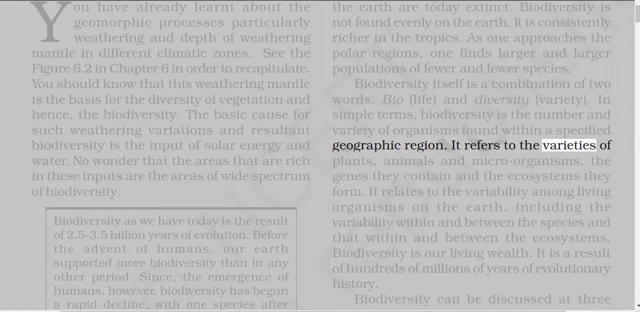 geographic region. It refers to the varieties of plants, animals and microorganisms, the genes they contain and the ecosystems they form. It relates to the variability among living organisms on the earth, including plants, animals and microorganisms. Biodiversity is our living wealth. 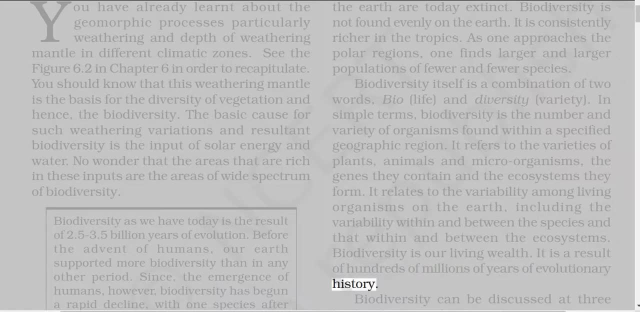 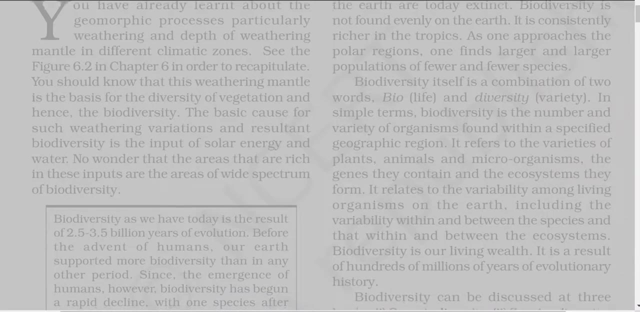 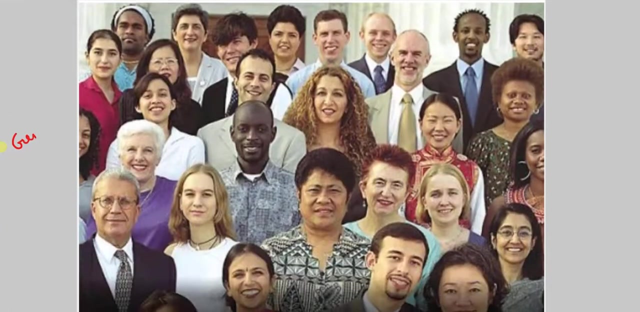 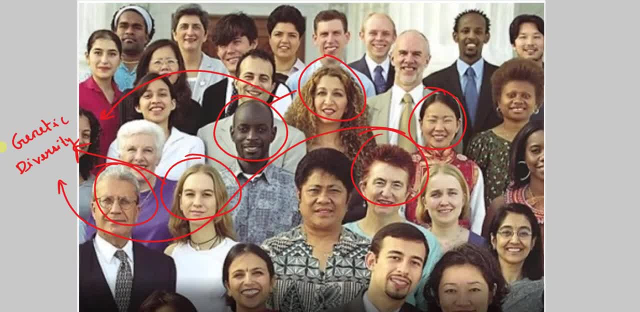 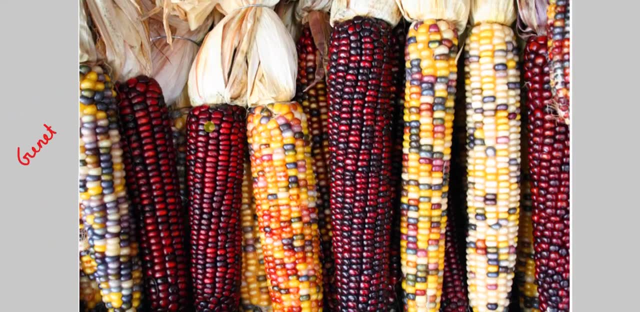 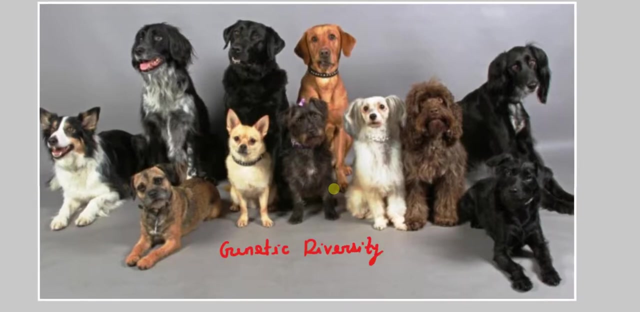 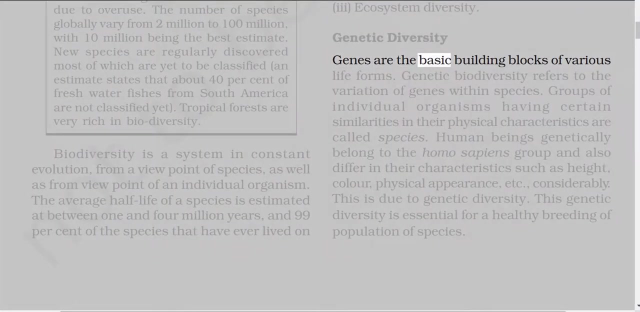 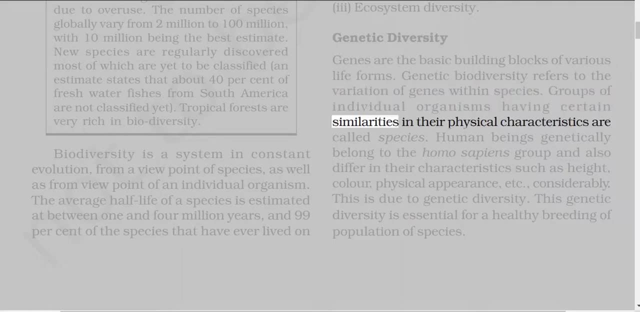 organisms having specific species in each. organisms having certain similarities in their physical characteristics are called species. Human beings genetically belong to the Homo sapiens group and also differ in their characteristics such as height, color, physical appearance etc. considerably. This is due to genetic diversity. This genetic diversity is essential. 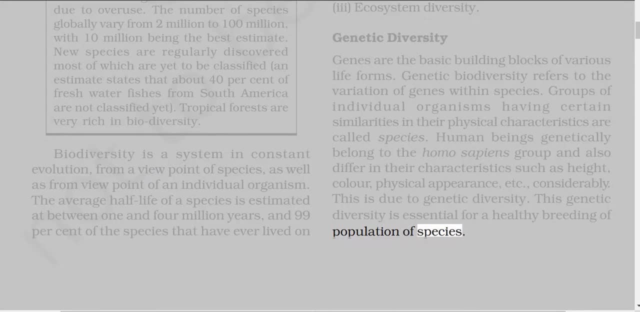 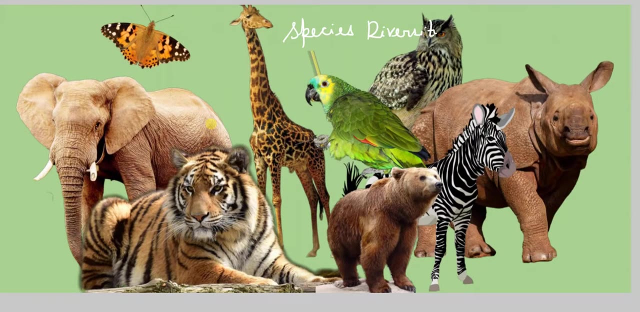 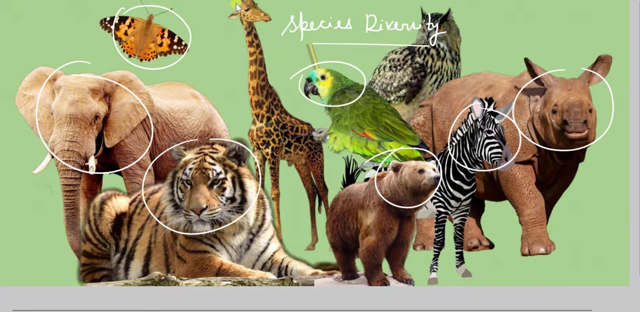 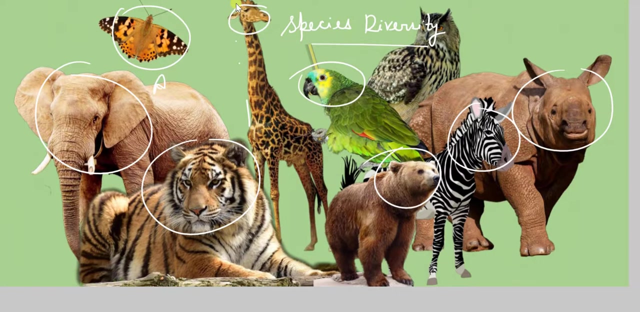 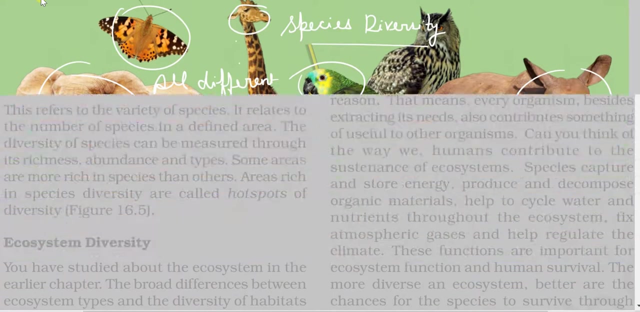 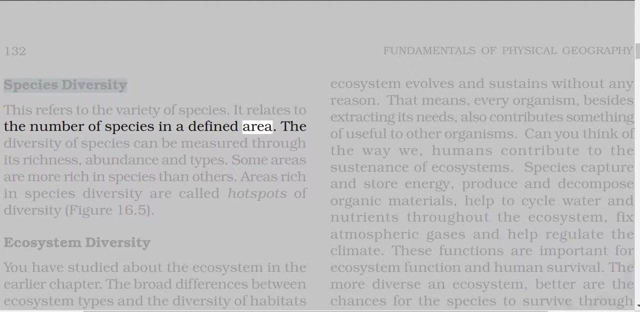 for a healthy breeding of population of species. Species Diversity: This refers to the variety of species. It relates to the number of species in a defined area. The diversity of species để khác: tinh thùng csg của chính cải, tr Hankge. hà dứt tenim tính n medios diện tình xang ngseason năng trường kiến đjob. This refers to the variety of species. It relates to the number of species in a defined area, Theinent ofů. 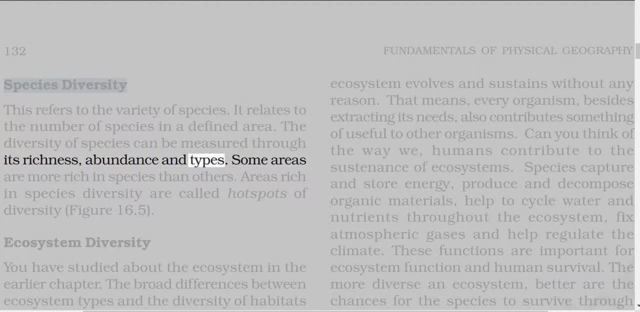 species who fingersert never aljareá body of species. öt customers men дор gKSeany by breakthrough of species. dai DPیں nhatched. some duùng species can be measured through its richness, abundance and types. Some areas are more rich. 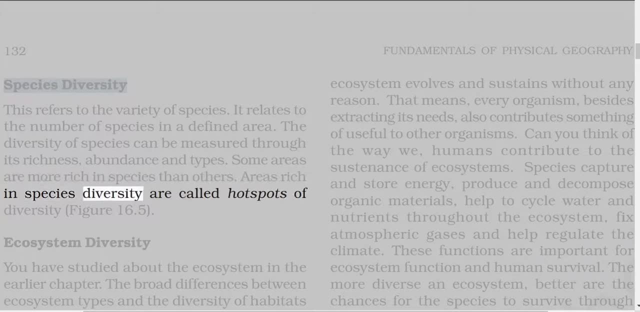 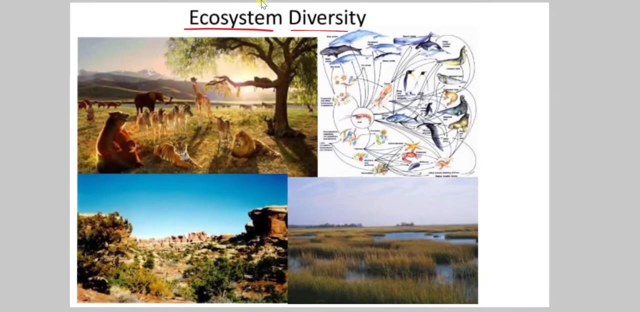 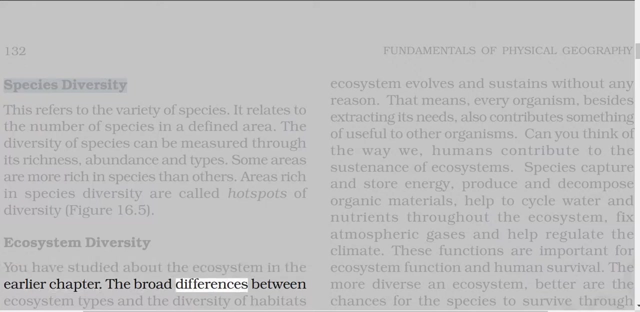 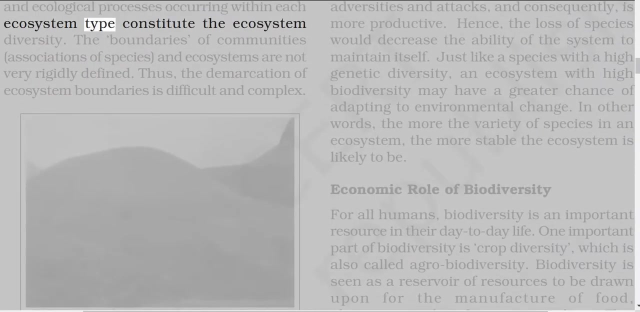 in species than others. Areas rich in species diversity are called hotspots of diversity. Ecosystem diversity: You have studied about the ecosystem in the earlier chapter. The broad differences between ecosystem types and the diversity of habitats and ecological processes occurring within each ecosystem type constitute the ecosystem diversity. 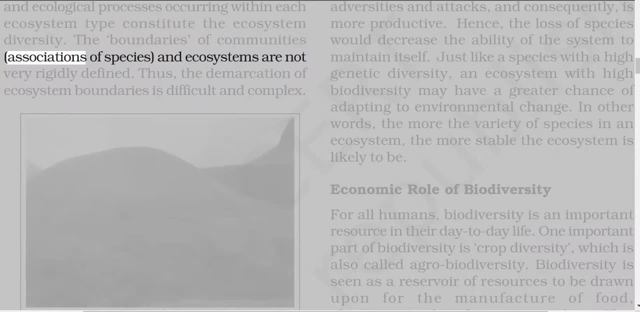 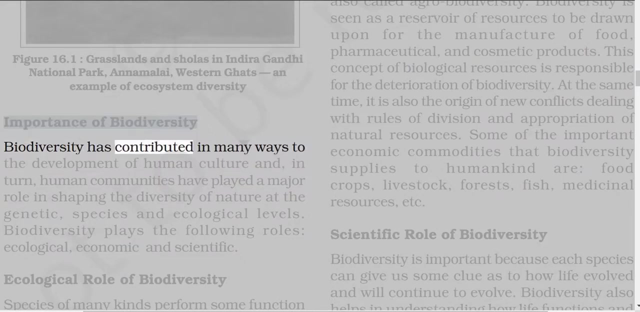 The boundaries of communities, associations of species and ecosystems are not very rigidly defined. Thus the demarcation of ecosystem boundaries is difficult and complex. Importance of Biodiversity. Biodiversity has contributed in many ways to the development of human culture and, in turn, 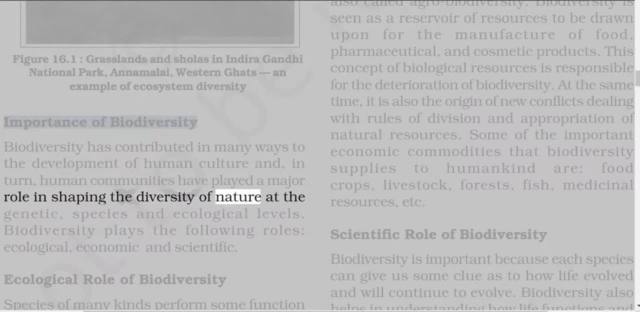 human communities have played a major role in shaping the diversity of nature at the genetic, species and ecological levels. Biodiversity plays the following role: Biodiversity plays the following role: Ecological, Economic and Scientific. Ecological role of Biodiversity. 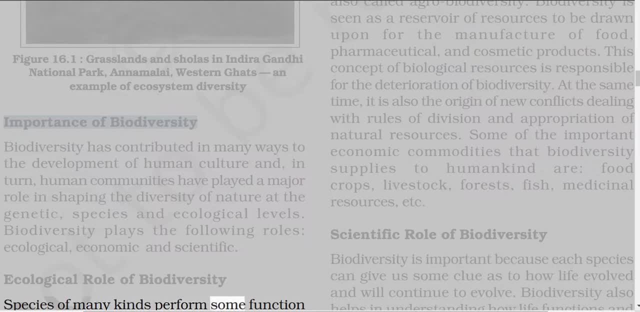 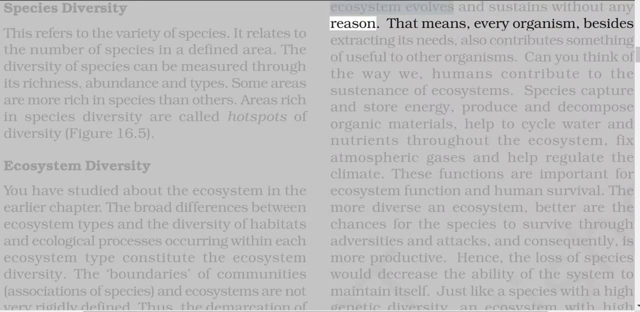 Species of many kinds perform some function or the other in an ecosystem. Nothing in an ecosystem evolves and sustains without any reason. That means every organism, besides extracting its needs, also contributes something of useful to other organisms. Can you think of the way we humans contribute to the sustenance of ecosystems? 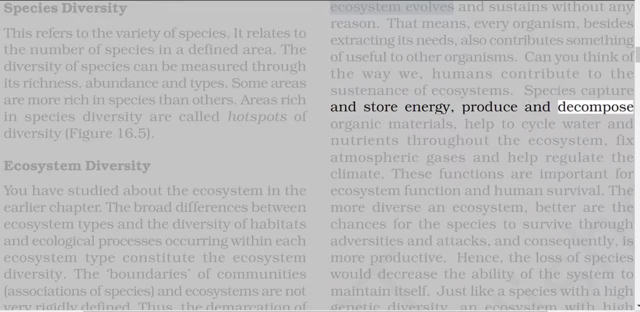 Species capture and store energy, produce and decompose organic materials, help to cycle water and nutrients throughout the ecosystem, fix atmospheric gases and help regulate the climate. These functions are important for ecosystem function and human survival. The more diverse an ecosystem, better are the chances for the species to survive through. 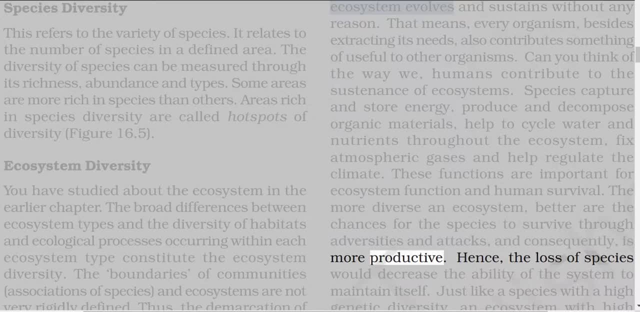 adversities and attacks and consequently, is more productive. Hence the loss of species would decrease the ability of the system to maintain and survive. The more diverse an ecosystem, the better it is to maintain itself, Just like a species with a high genetic diversity, an ecosystem with high 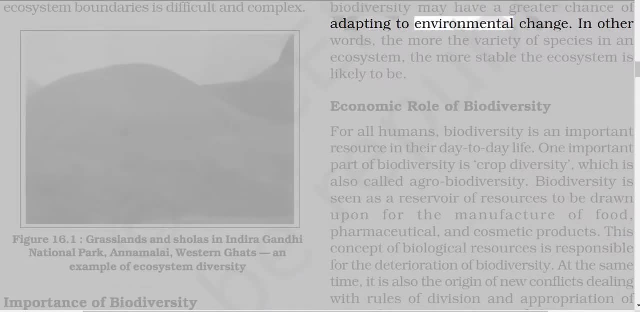 biodiversity may have a greater chance of adapting to environmental change. In other words, the more the variety of species in an ecosystem, the more stable the ecosystem is likely to be. Economic role of Biodiversity. For all humans, biodiversity is an important resource in their day-to-day life. 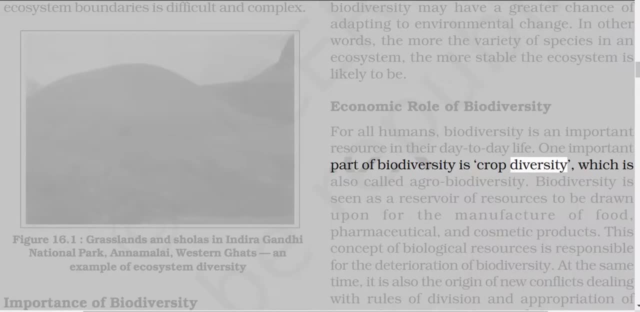 One important part of biodiversity is crop diversity, which is also called agrobiodiversity. Biodiversity is seen as a reservoir of resources to be drawn upon for the manufacture of food, pharmaceutical and cosmetic products. This concept of biological resources is responsible for the deterioration of biodiversity. 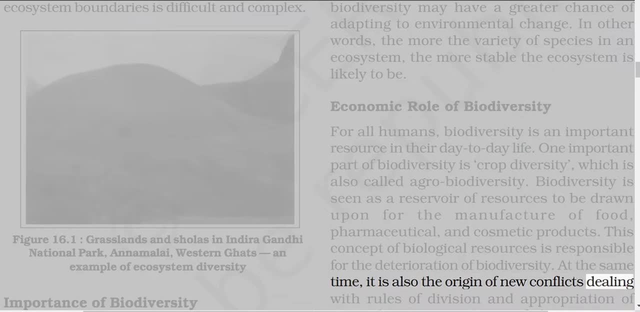 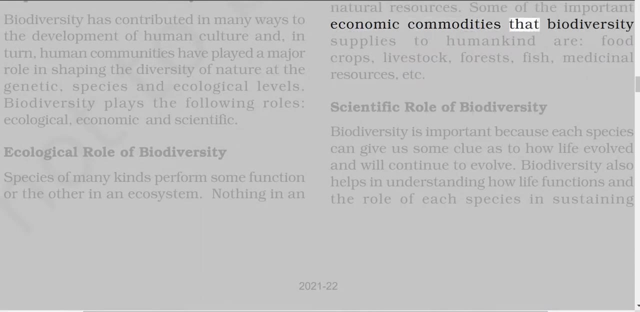 At the same time, it is also the origin of new conflicts dealing with rules of division and appropriation of natural resources. Some of the important economic commodities that biodiversity is responsible for are food, natural resources and natural resources. Biodiversity is also the source of food, natural resources and natural resources. Biodiversity supplies to humankind are: 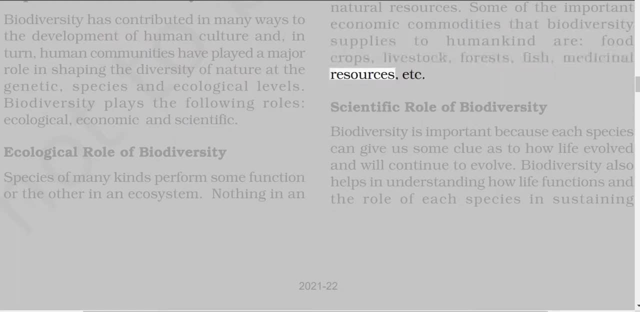 food crops, livestock, forests, fish, medicinal resources, etc. Scientific role of Biodiversity. Biodiversity is important because each species can give us some clue as to how life evolved and will continue to evolve. Biodiversity also helps in understanding how life functions. 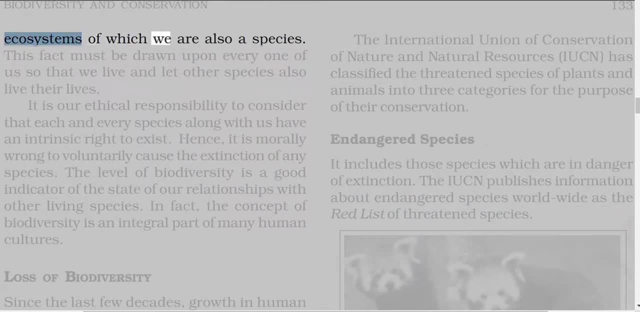 and the role of each species in sustaining ecosystems, of which we are also a species. This fact must be drawn upon every one of us so that we live and let other species also live their lives. It is our ethical responsibility to consider that each and every species, along with us, have an 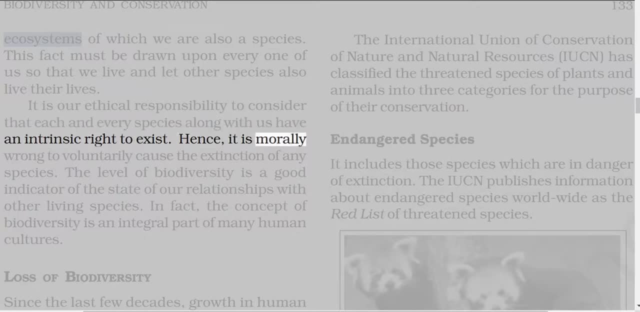 intrinsic right to exist. Hence it is morally wrong to voluntarily cause the extinction of any species. The level of biodiversity is a good indicator of the state of our relationships with other living species. In fact, the concept of biodiversity is an integral part of many. 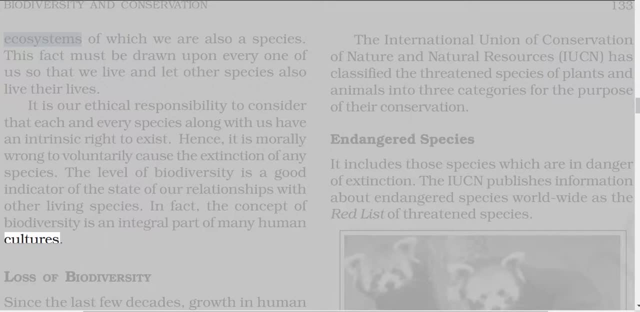 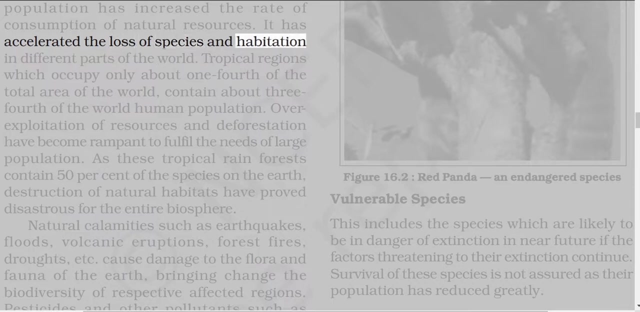 human cultures: Loss of Biodiversity. Since the last few decades, growth in human population has increased the rate of consumption of natural resources. It has accelerated the loss of species and habitation in different parts of the world, Tropical regions, which occupy only about one-fourth of the total area of the world. 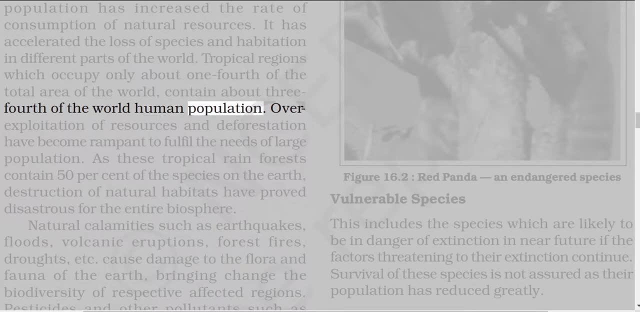 contain about three-fourth of the world human population. Overexploitation of resources and deforestation have become rampant to fulfill the needs of large population. As these tropical rain forests contain 50% of the species on the earth, destruction of natural habitats have proved disastrous for the entire biosphere. Natural calamities such as earthquakes, 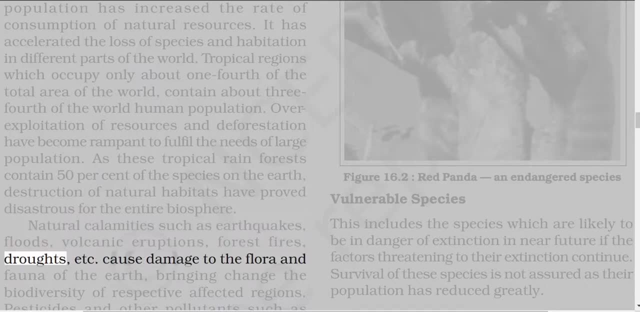 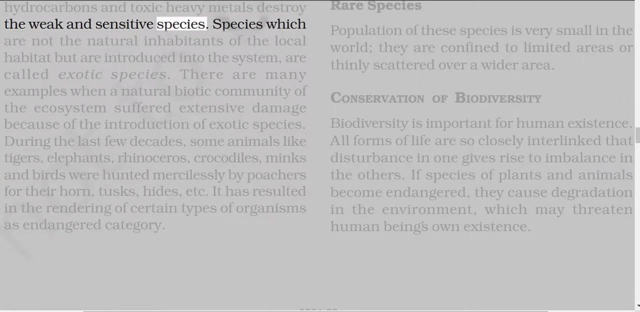 floods, volcanic eruptions, forest fires, droughts, etc. cause damage to the flora and fauna of the earth, bringing change the biodiversity of respective affected regions. Pesticides and other pollutants, such as hydrocarbons and toxic heavy metals, destroy the weak and sensitive species, Species which are not the natural inhabitants of the local habitat. 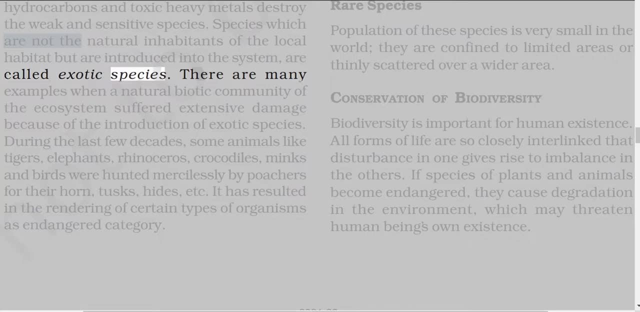 but are introduced into the system are called exotic species. There are many examples when a natural biotic community of the ecosystem suffered extensive damage because of the introduction of exotic species During the last few decades. some animals like tigers, elephants, rhinoceros, 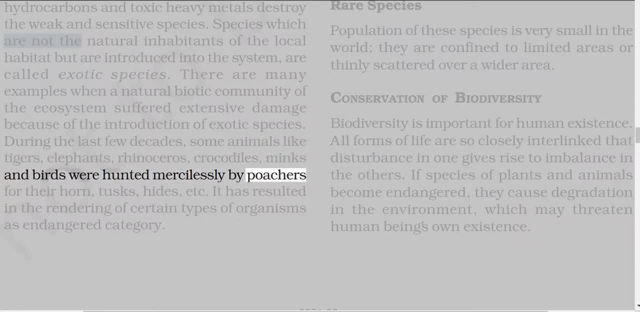 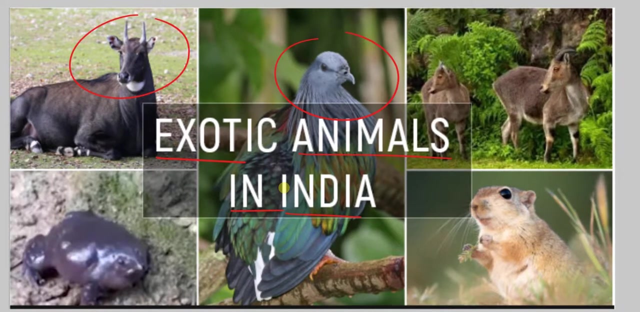 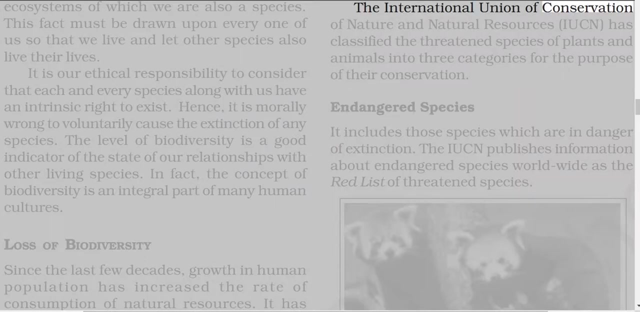 crocodiles, minks and birds were hunted mercilessly by poachers for their horn, tusks, hides, etc. It has resulted in the rendering of certain types of organisms as endangered category. The International Union of Conservation of Nature and Natural Resources has 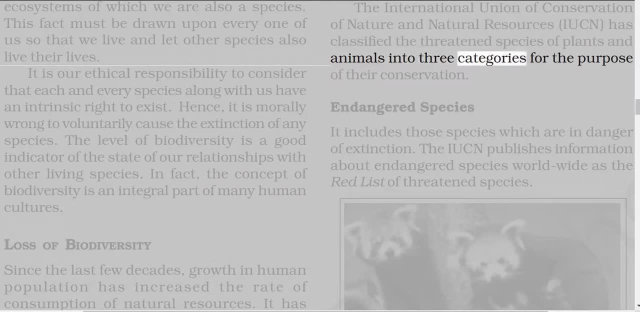 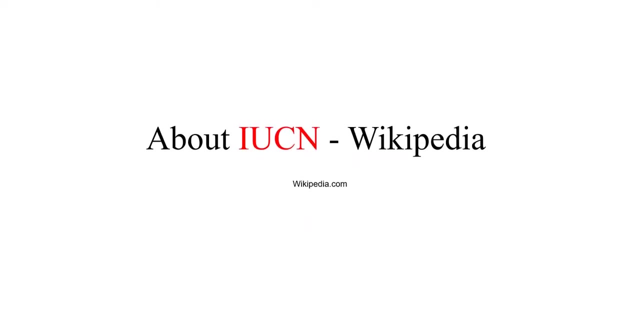 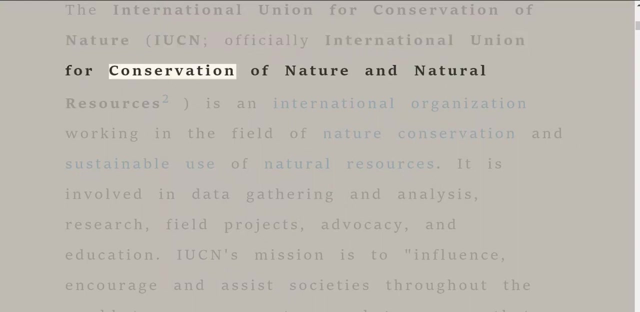 classified the threatened species of plants and animals into three categories for the purpose of their conservation: The International Union for Conservation of Nature- Officially International Union for Conservation of Nature and Natural Resources, IUCN 19,. the national organisation working in the field of nature conservation. and. 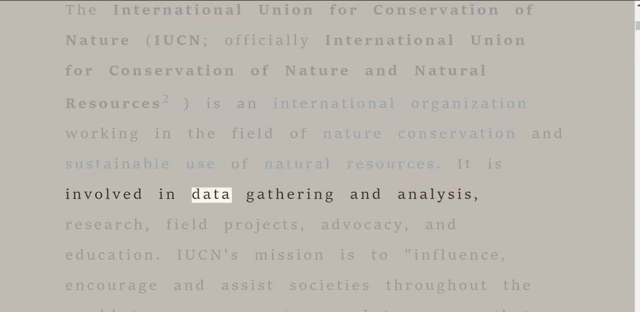 use of natural resources. It is involved in data gathering and analysis, research, field projects, advocacy and education. IUCN's mission is to influence, encourage and assist societies throughout the world to conserve nature and to ensure that any use of natural 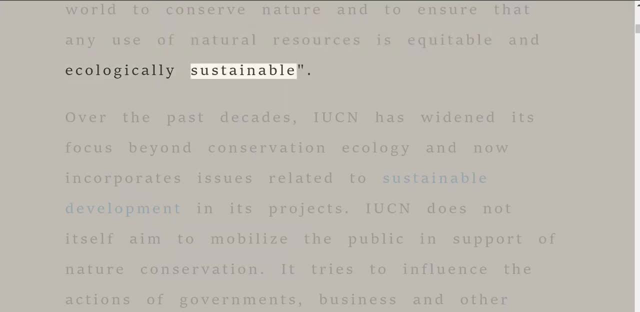 resources is equitable and ecologically sustainable. Over the past decades, IUCN has widened its focus beyond conservation ecology and now incorporates issues related to sustainable development in its projects. IUCN does not itself aim to mobilize the public in support of nature. 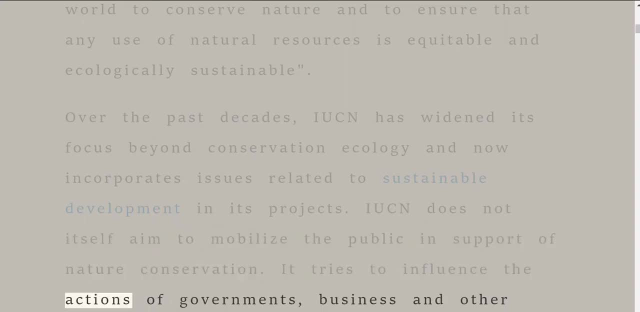 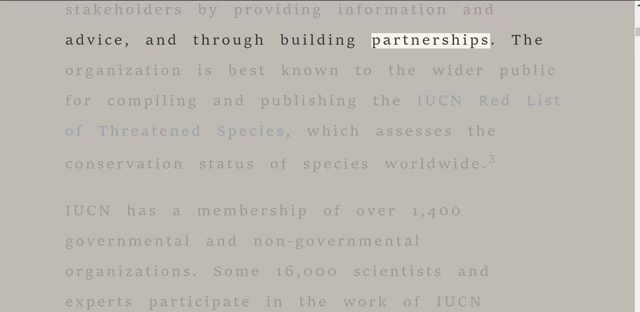 conservation. It tries to influence the actions of governments, business and other stakeholders by providing information and advice and through building partnerships. The organization is best known to the wider public for compiling and publishing the IUCN Red List of Threatened Species, which assesses the importance of conservation and conservation of nature. 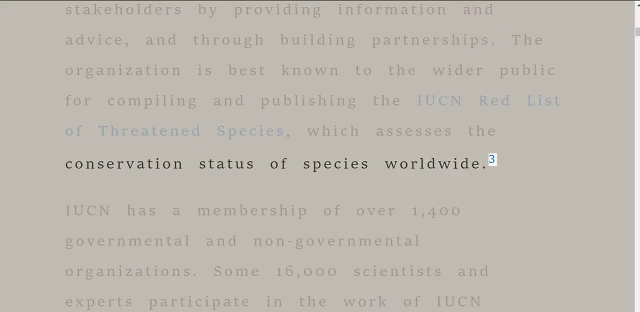 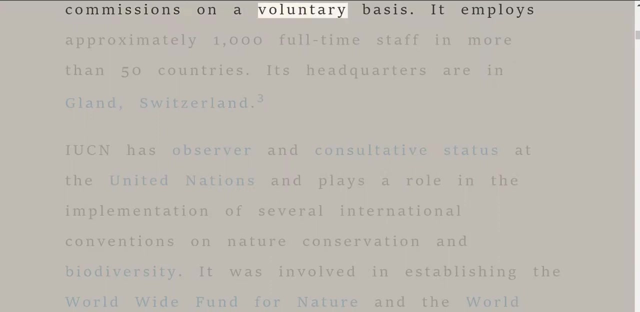 The IUCN Red List of Threatened Species, which assesses the conservation status of species worldwide. IUCN has a membership of over 1,400 governmental and non-governmental organizations. Some 16,000 scientists and experts participate in the work of IUCN commissions on a voluntary 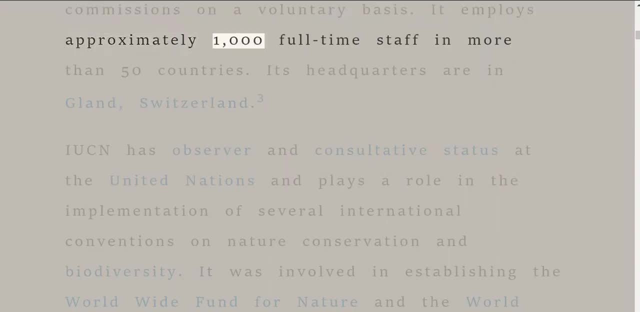 basis. It employs approximately 1,000 full-time staff in more than 50 countries. Its headquarters are in Gland, Switzerland. IUCN has observer and consultative status at the United Nations and plays a role in the implementation of several international conventions on nature conservation and biodiversity. It was involved in establishing 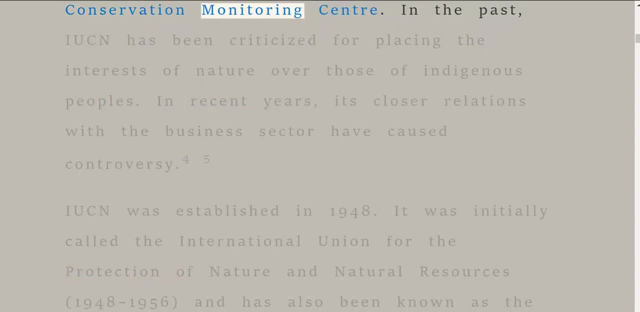 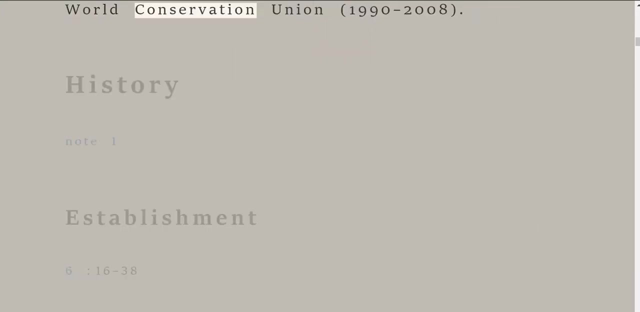 the World Wide Fund for Nature and the World Conservation Monitoring Center. In the past, IUCN has been criticized for placing the interests of nature over those of indigenous peoples. In recent years, its closer relations with the business sector have caused controversy. The partnership between the two countries is of cultural importance to the Kaito sandwiches. 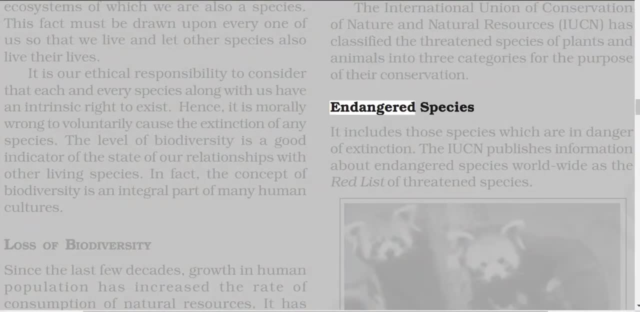 The IUCN Red List of Threatened Species, which it Cela wears six more times, has come to be ministered to arease development developments in Taiwan, The International Union of the Protection of Nature and Natural Resources. The International Union of the Protection of Nature and Natural Resources has become known in 1996 as WCU dev taking. 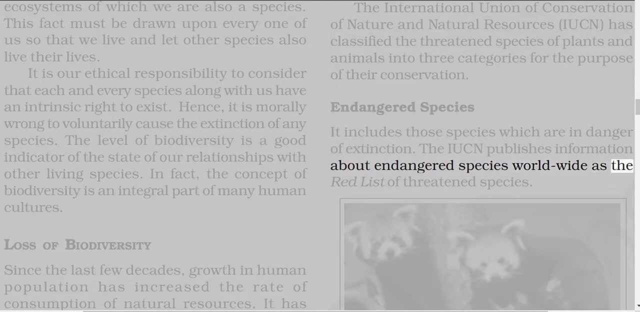 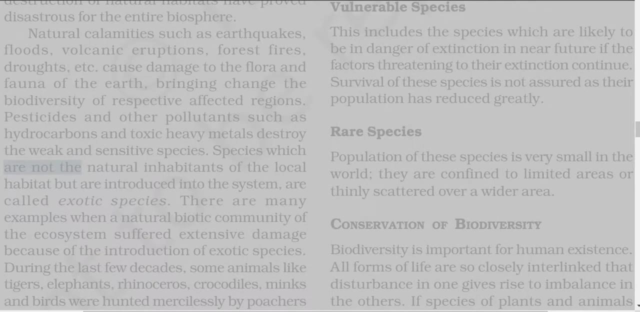 place in如此 World Conservation Union, creating many of the world's entrance in the World Conservation Union inward, which included Nicholas Bell and his colleagues Craig Kopges. Also, the United species worldwide as the red list of threatened species- Vulnerable species. This includes the species which are likely to be in danger of extinction in near future. 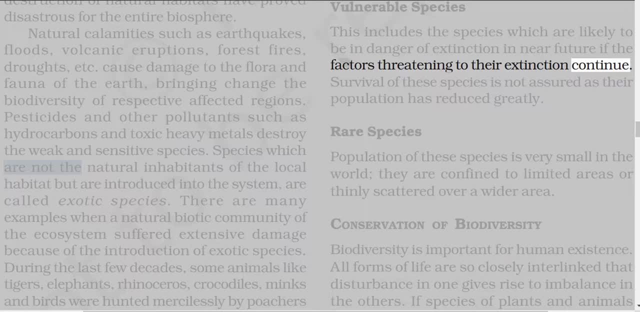 if the factors threatening to their extinction continue. Survival of these species is not assured, as their population has reduced greatly. Rare species Conservation of these species is very small in the world. they are confined to limited areas or thinly scattered over a wider area. 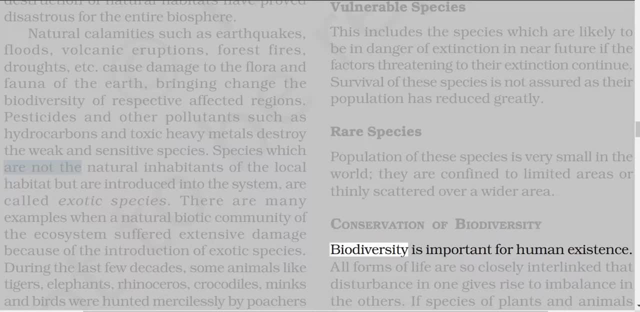 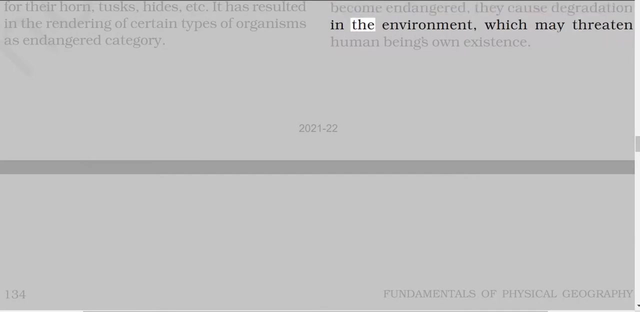 Conservation of biodiversity. Biodiversity is important for human existence. All forms of life are so closely interlinked that disturbance in one gives rise to imbalance in the others. If species of plants and animals become endangered, they cause degradation in the environment which may threaten human beings' own existence. 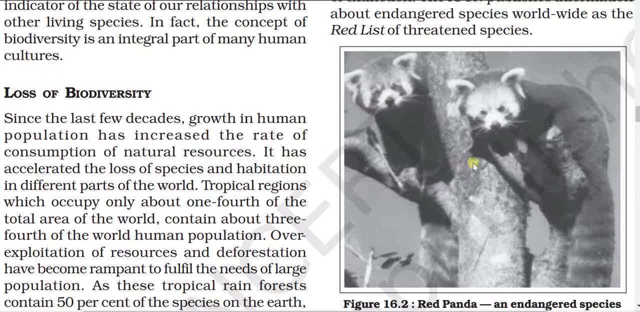 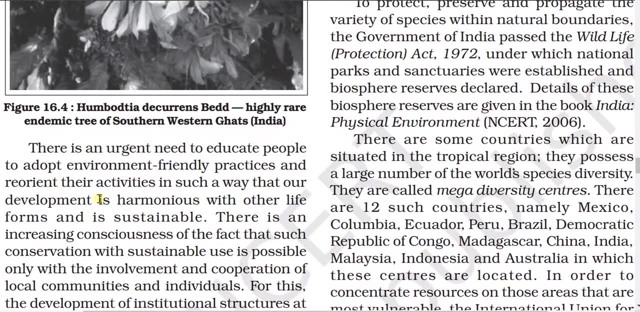 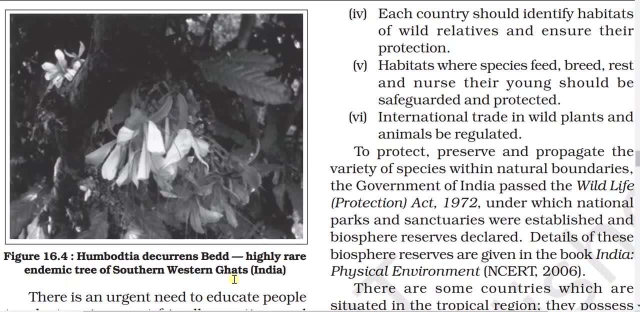 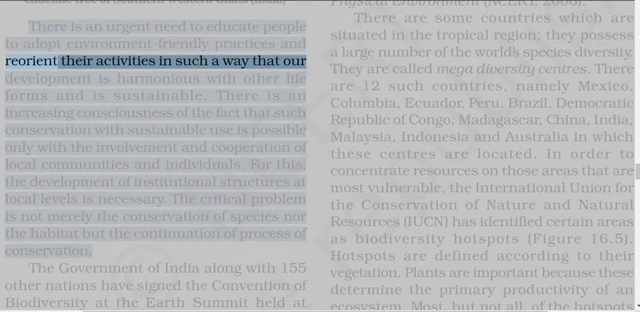 There is an urgent need to educate people to adopt environment-friendly practices and reorient their activities in such a way that our development is harmonious with other life forms and is sustainable. There is an increasing consciousness of the fact that such conservation with sustainable use is possible only with the involvement and cooperation of local communities and individuals. 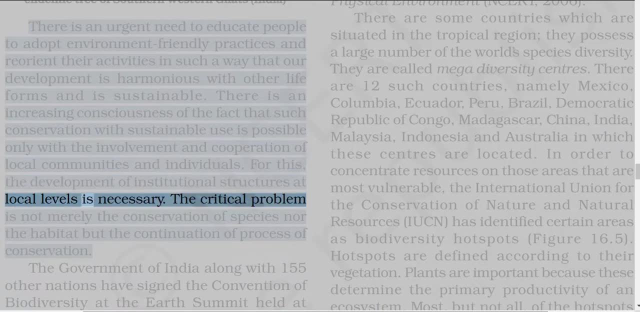 For this, the development of institutional structures at local levels is necessary. The critical problem is not merely the conservation of species nor the habitat, but the continuation of process of conservation. The Government of India, along with 155 other nations, have signed the Convention of Biodiversity. 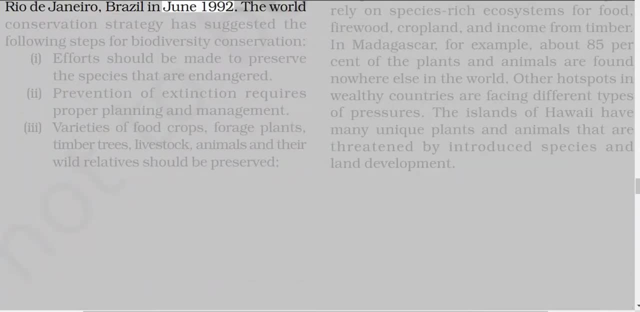 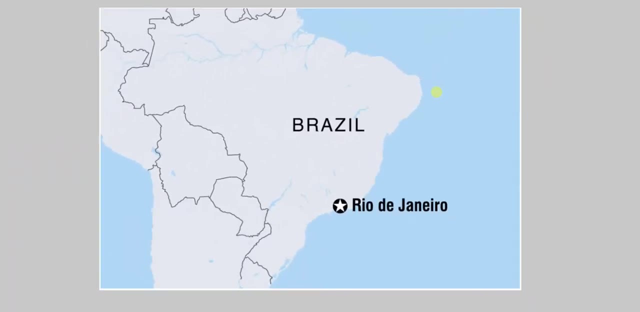 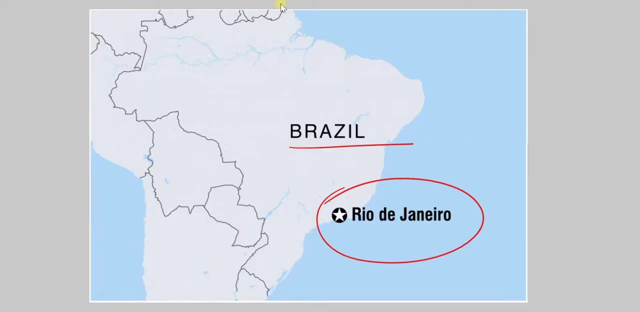 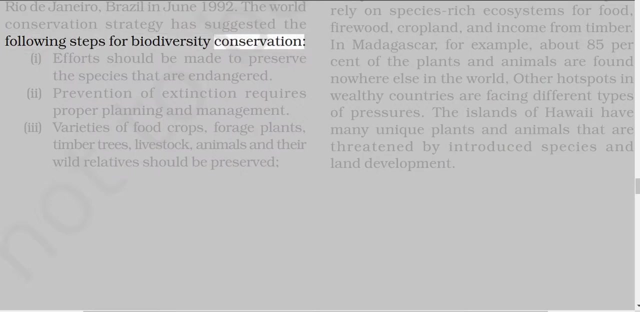 at the Earth Summit held at Rio de Janeiro, Brazil, in June 1992.. The World Conservation Strategy has suggested the following steps for biodiversity conservation: 1. Efforts should be made to preserve the species that are endangered. 2. Prevention of extinction requires proper planning and management. 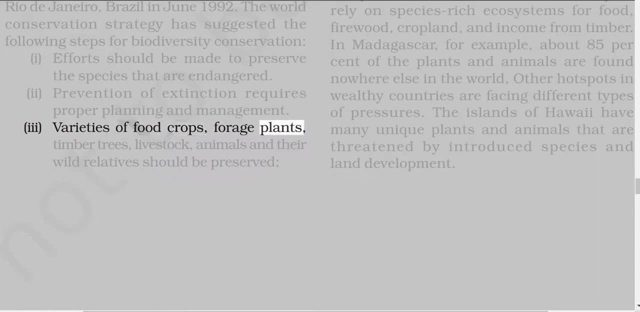 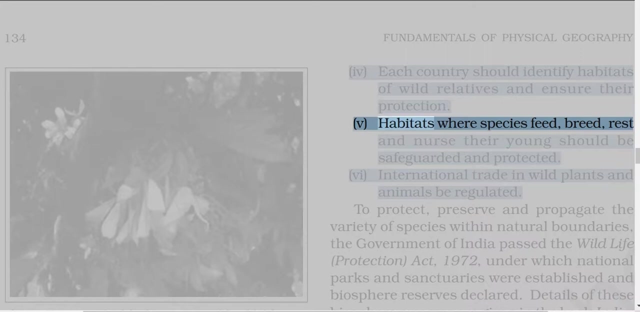 3. Varieties of food crops, forage plants, timber trees, livestock animals and their wild relatives should be preserved. 4. Each country should identify habitats of wild relatives and ensure their protection. v Habitats where species feed, breed, rest and nurse their young should be safeguarded. 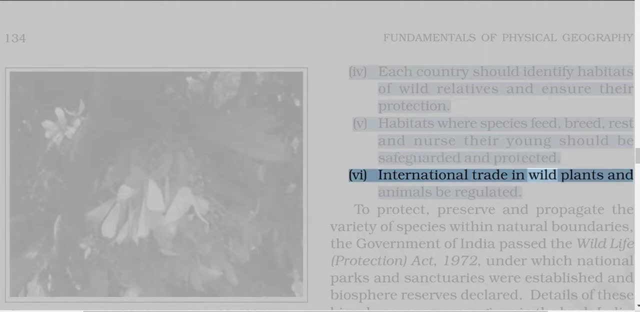 and protected. 6. International trade in wild plants and animals be regulated To protect, preserve and propagate the variety of species within natural boundaries. the Government of India passed the Wildlife Protection Act 1972, under which national parks and sanctuaries were established and biosphere reserves declared. 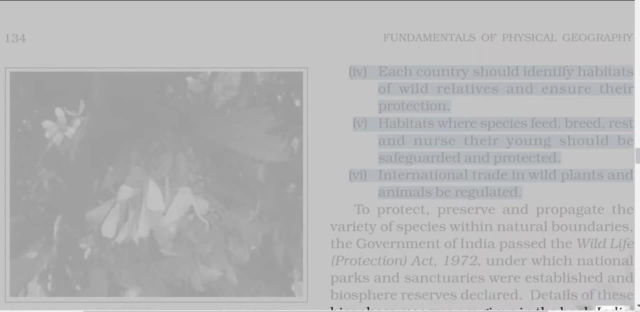 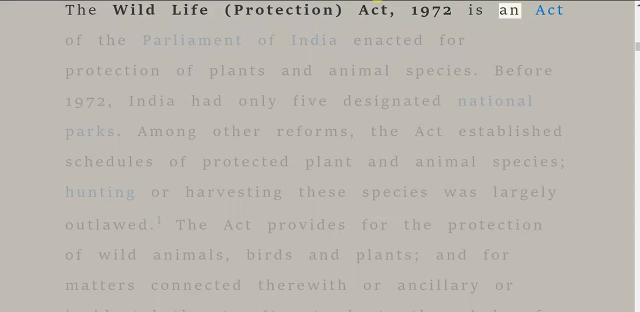 Details of these biosphere reserves are given in the book India Physical Environment, insert 2006.. The Wildlife Protection Act 1972, is an act of the Parliament of India enacted for protection of plants and animal species. Before 1972, India had only five designated national. 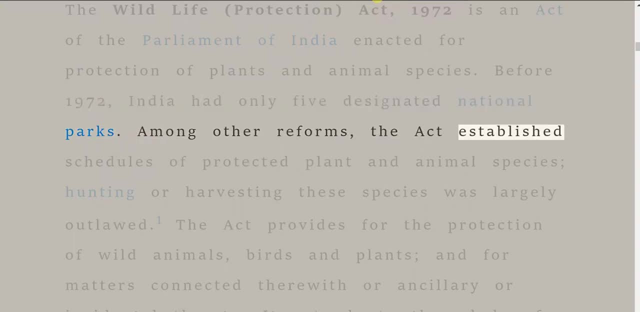 parks. Among other reforms, the Act established schedules of protected plant and animal species. hunting or harvesting these species was largely outlawed. The Act provides for the protection of wild animals, birds and plants and for matters connected therewith or ancillary or incidental thereto. It extends to the whole of India. 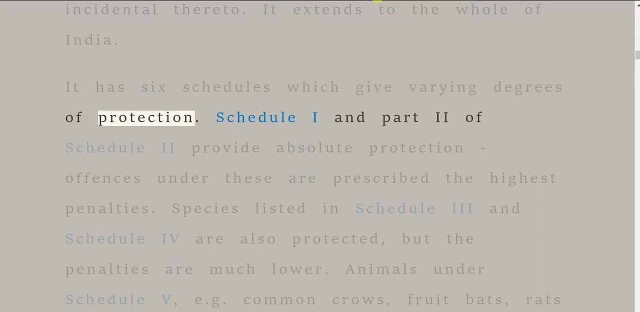 It has six schedules which give varying degrees of protection. Schedule I and Part II of Schedule II provide absolute protection of fences. under these are prescribed the highest level of protection. Schedule II and Part II of Schedule II provide absolute protection of fences. under these are prescribed the highest level of protection. 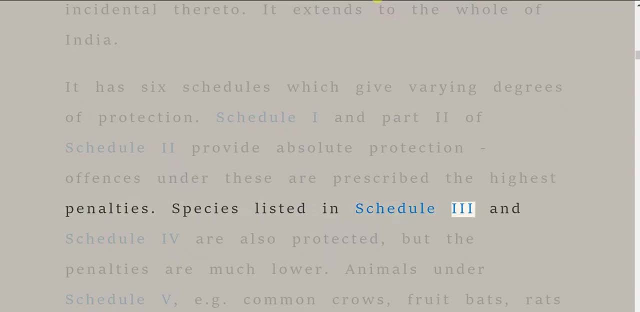 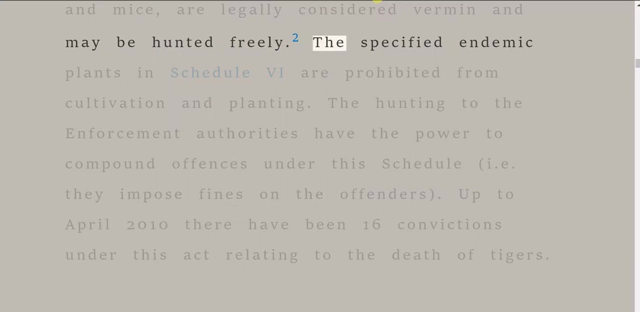 Species listed in Schedule III and Schedule IV are also protected, but the penalties are much lower. Animals under Schedule V- eg common crows, fruit bats, rats and mice- are legally considered vermin and may be hunted freely. The specified endemic plants in Schedule VI are prohibited from cultivation and planting. 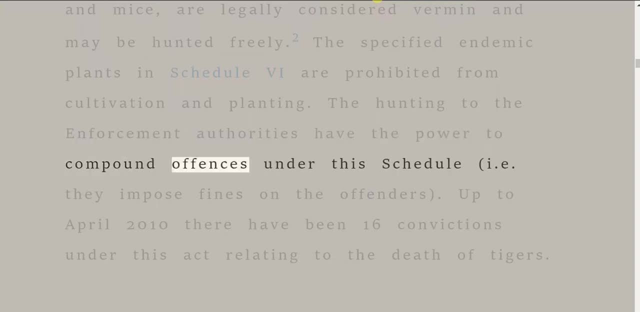 The hunting to the enforcement authorities have the power to compound offenses under this schedule, ie they impose fines on the enforcement authorities. Up to April 2010, there have been 16 convictions under this Act relating to the death of tigers. History. 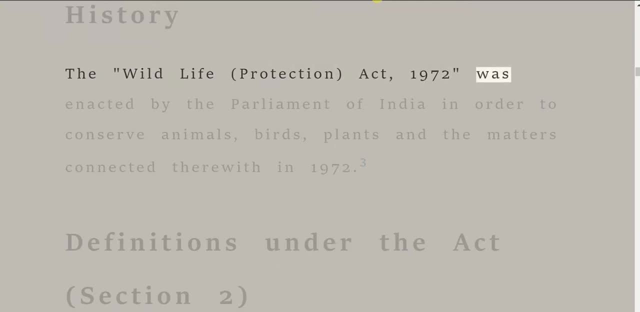 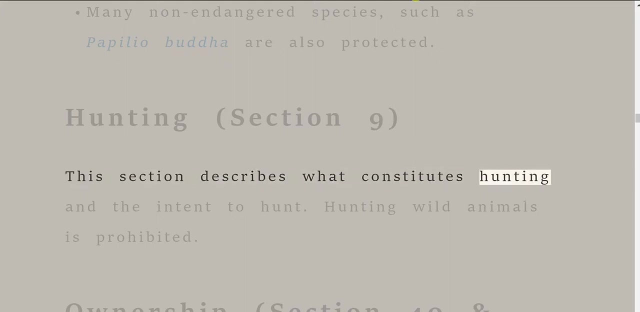 The Wildlife Act 1972 was enacted by the Parliament of India in order to conserve animals, birds, plants and the matters connected therewith in 1972.. Hunting- Section 9. This section describes what constitutes hunting and the intent to hunt. 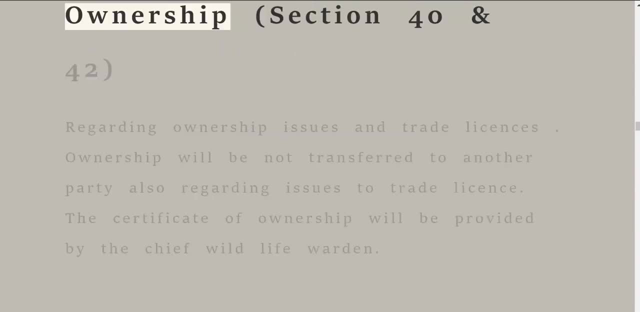 Hunting wild animals is prohibited. Section 40 and 42: Regarding ownership issues and trade licenses: Ownership will be not transferred to another party. also, regarding issues to trade license, The Certificate of Ownership will be provided by the chief wildlife warden. Section 51: 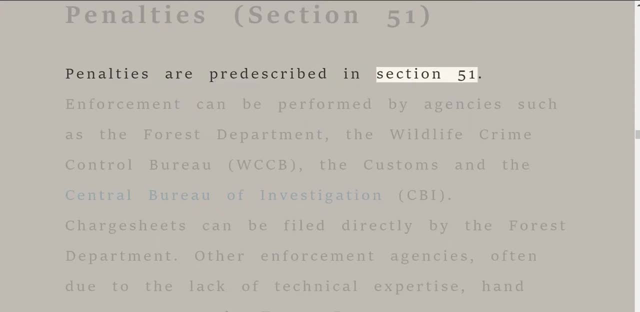 Penalties are pre-described in Section 51.. Enforcement can be conducted and avoided performed by agencies such as the forest department, the wildlife crime control bureau, wccb, the customs and the central bureau of investigation, cbi. charge sheets can be filed directly by the forest department. other enforcement agencies, often due to the lack of technical. 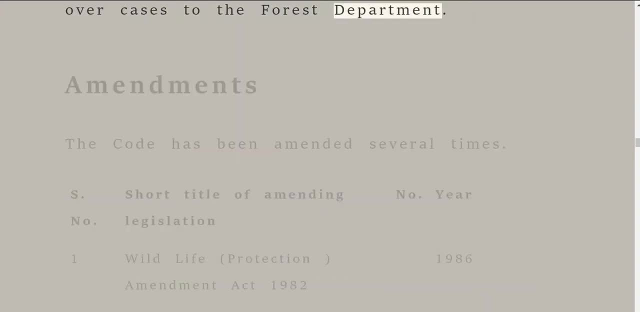 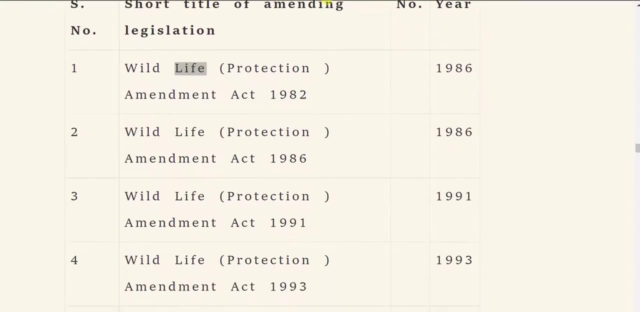 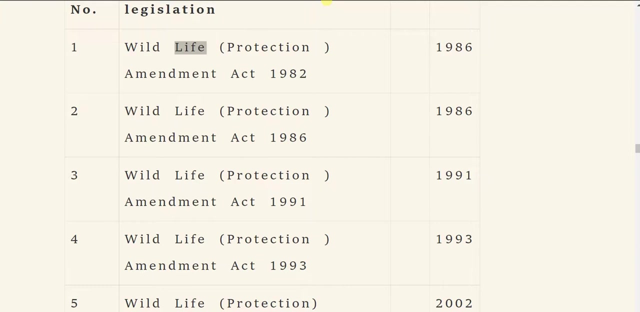 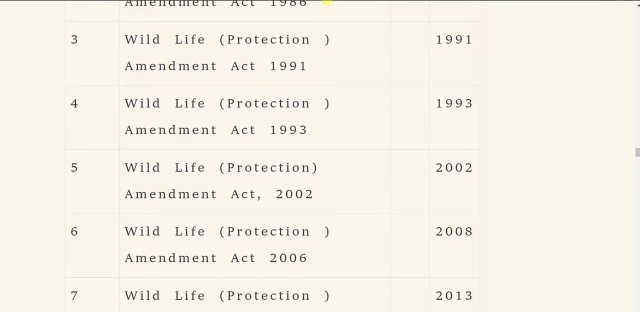 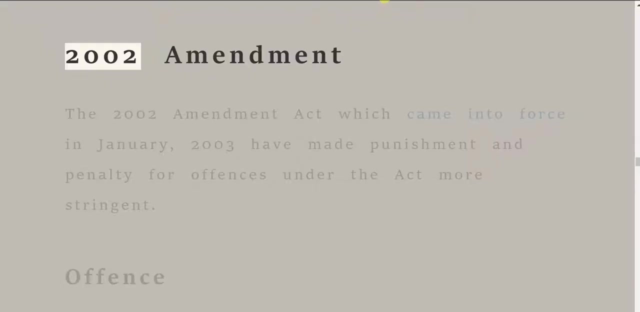 expertise hand over cases to the forest department. amendments: the code has been amended several times, so 2002 amendment: the 2002 amendment act, which came into force in january 2003, have made punishment and penalty for offenses under the act more stringently: offense for offenses relating to wild animals or their parts and products included in schedule i or 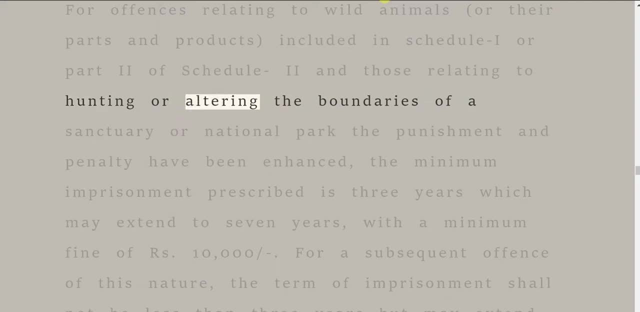 part 2 of schedule 2 and those relating to hunting or altering the boundaries of a sanctuary or national park. the punishment and penalty have been enhanced. the minimum imprisonment prescribed is three years, which may extend to seven years, with a minimum fine of rs 10 000. slash dash. 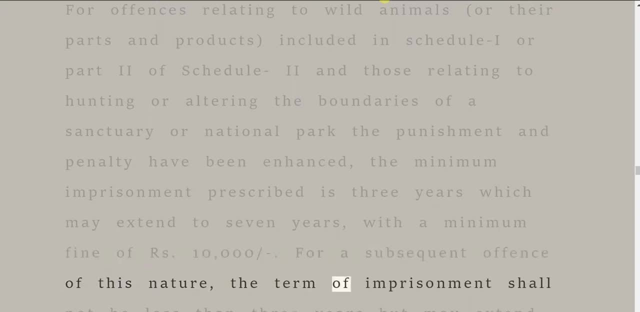 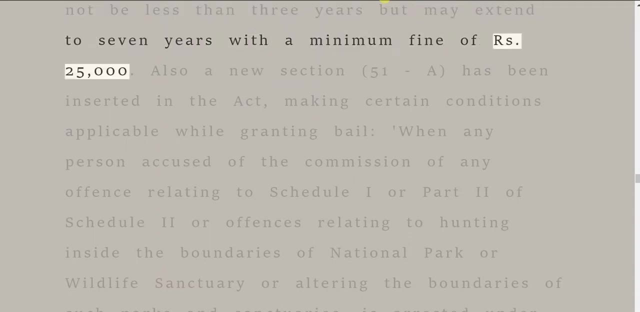 for a subsequent offense of this nature, the term of imprisonment shall not be less than three years, but may extend to seven years, with a minimum fine of 25 000 rupees. also, a new section 51a has been inserted in the act, making certain conditions applicable, while 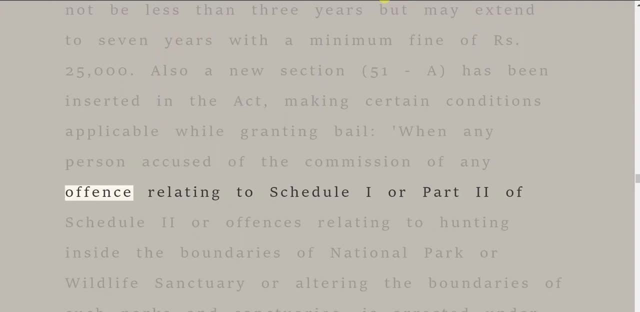 granting bail when any person accused of the commission of any offense relating to schedule i or part 2 of schedule 2, or offenses relating to hunting inside the boundaries of national park or wildlife sanctuary or wildlife sanctuary, or altering the boundaries of such parks and sanctuaries, is arrested under the provisions of. 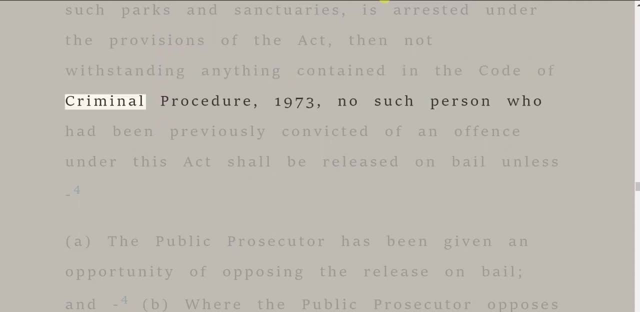 the act than, notwithstanding anything contained in the code of criminal procedure 1973, no such person, who had been previously convicted of an offense under this act, shall be released on bail unless a. the public prosecutor has been given an opportunity of opposing the release on bail, and minus 4b, where the public prosecutor opposes the application. the court is satisfied that there 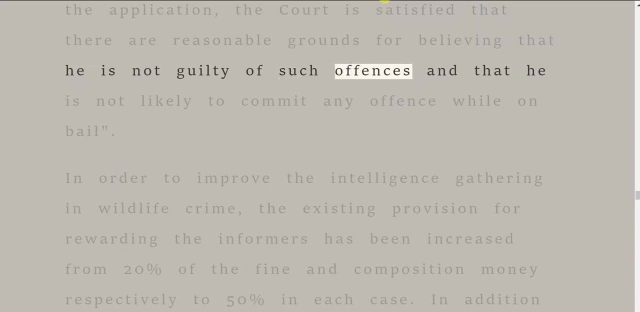 are reasonable grounds for the application of the code of criminal procedure. yet that such a bill should be accepted in light of a case whether it was disclosed by the system, gosh, that's wrong. it is very probably not the case. instead, he is not held responsible and bail file land and educational ᵗᵉ� eiᵉᵐᵉᵒᵂ. 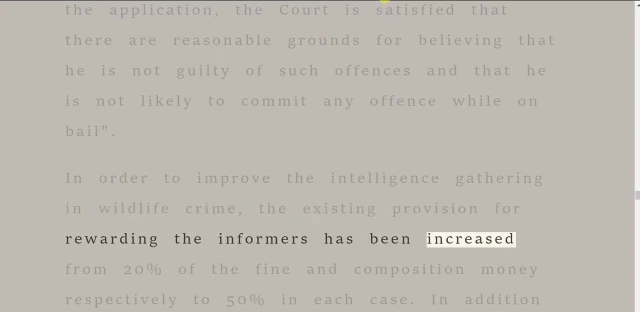 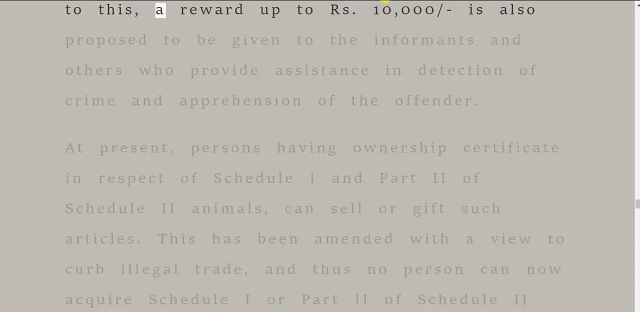 has been such Information in the form such cases and for something that can even be mystical, so that there are no evidences that he may have committed offenses on bail and that he is not likely to commit any offense while on bail. in order to improve the intelligence gathering and wildlife crime, the existing provision for rewarding the informers has been increased from 20% of the fine and composition money respectively to 50% in each case. in addition to this, a reward up to our s 10 00 0 pa is also proposed to be given to the informants and others who provide assistance in detection of crimes which are agora. 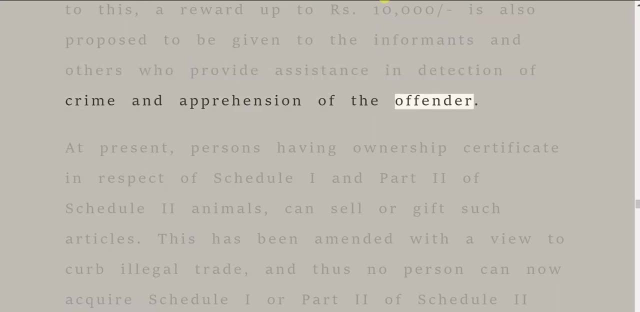 we're getting off camera in detection of crime and apprehension of the offender. At present, persons having ownership certificate in respect of Schedule I and Part 2 of Schedule II- animals can sell or gift such articles. This has been amended with a view to curb illegal trade and thus no person can now 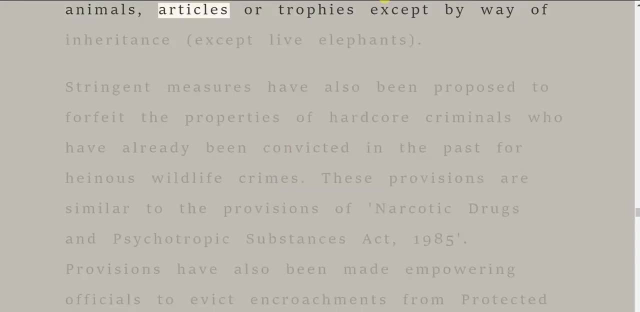 acquire Schedule I or Part 2 of Schedule II animals, articles or trophies, except by way of inheritance, except live elephants. Stringent measures have also been proposed to forfeit the properties of hardcore criminals who have already been convicted in the past for heinous wildlife. 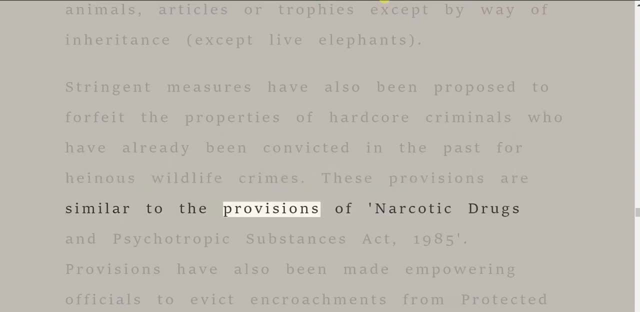 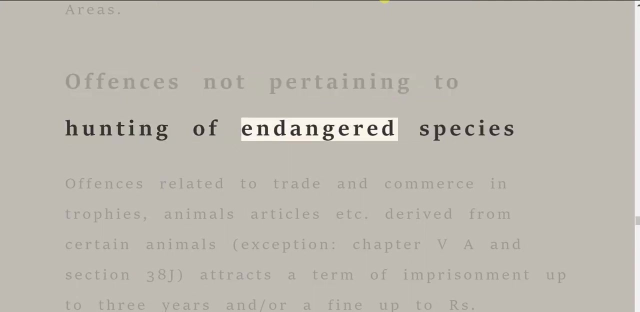 crimes. These provisions are similar to the Provisions of Narcotic Drugs and Psychotropic Substances Act 1985. Provisions have also been made empowering officials to evict encroachments from protected areas, Offenses Not Pertaining to Hunting of Endangered Species. 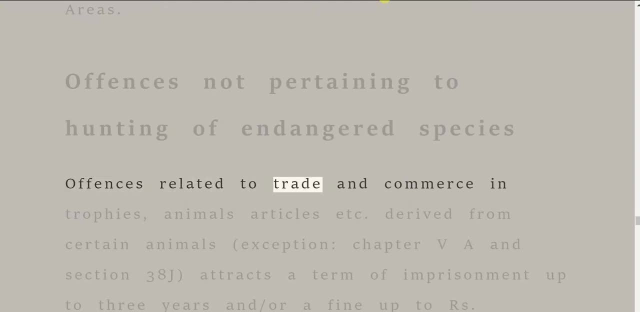 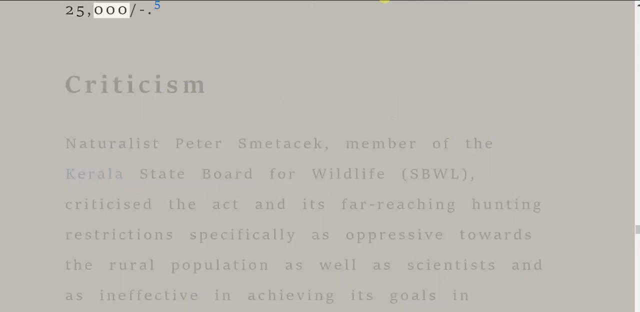 Offenses related to trade and commerce in trophies, animals' articles etc. derived from certain animals. exception Chapter 5A and Section 38J attracts a term of imprisonment up to three years and or a fine up to Rs 25,000-.5.. Criticism: 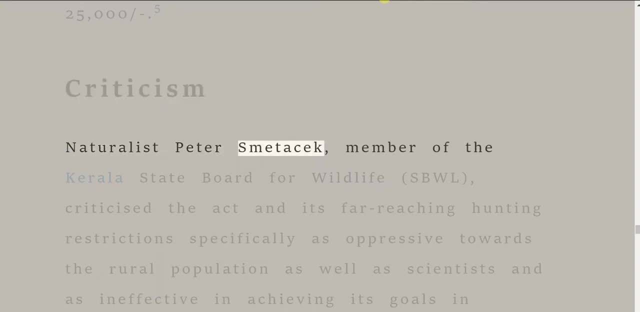 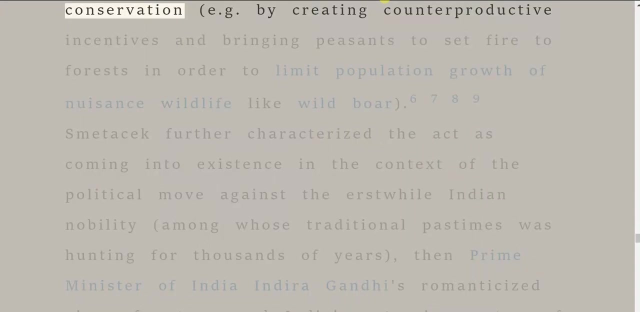 Naturalist Peter Smetasek, member of the Carroll Estate Board for Wildlife, SBWL, criticized the Act and its far-reaching hunting restrictions specifically as oppressive towards the rural population as well as scientists. It is ineffective in achieving its goals in conservation, eg by creating counterproductive. 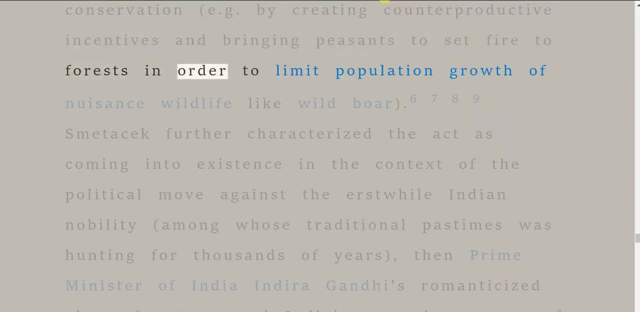 incentives and bringing peasants to set fire to forests in order to limit population growth of nuisance wildlife like wild boar. Smetasek further characterized the Act as coming into existence in the context of the political move against the erstwhile Indian nobility, among whose traditional pastimes was hunting for thousands of years then Prime. 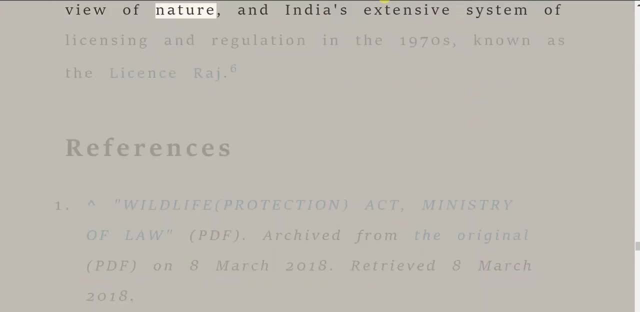 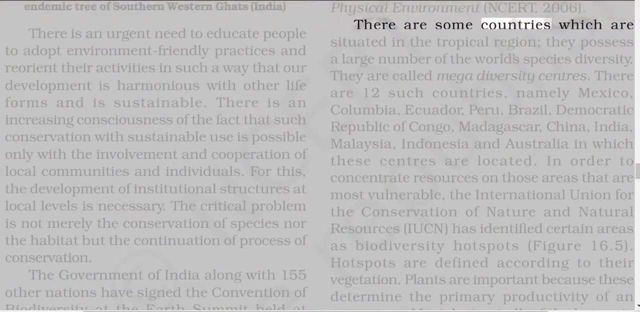 Minister of India Indira Gandhi's romanticized view of nature and India's extensive system of licensing and regulation in the 1970s, known as the License Raj. There are some countries which are situated in the tropical region. they possess a large number of the world's species diversity. They are called mega-diversity. 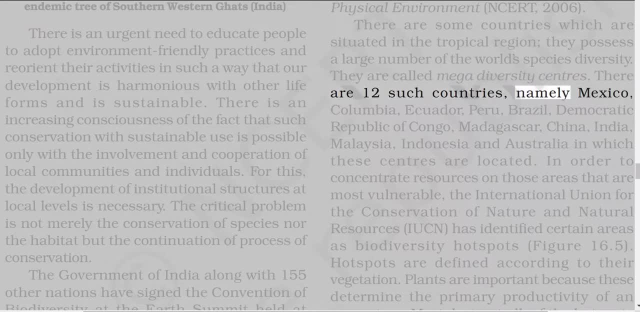 centers. There are 12 such countries, namely Mexico, Colombia, Ecuador, Peru, Brazil, Democratic Republic of Congo, Madagascar, China, India, Malaysia, Indonesia and Australia, in which many are located, In order to concentrate resources on those areas that are most vulnerable. 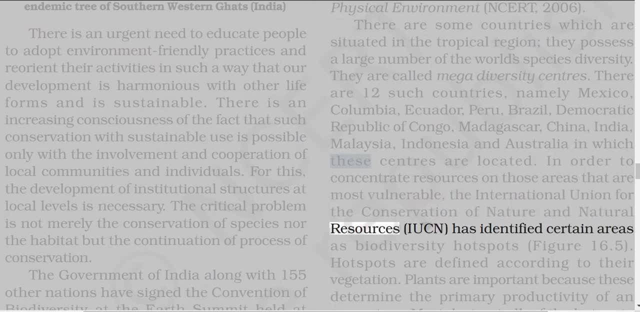 the International Union for the Conservation of Nature and Natural Resources has identified certain areas as biodiversity hotspots. Hotspots are defined according to their vegetation. Plants are important because these determine the primary productivity of an ecosystem. Most, but not all, of the hotspots rely on. 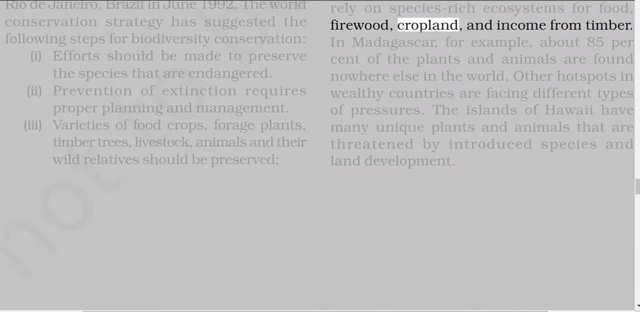 species-rich ecosystems for food, firewood crops and food and, of course, for consumption, wood cropland and income from timber. In Madagascar, for example, about 85% of the plants and animals are found nowhere else.